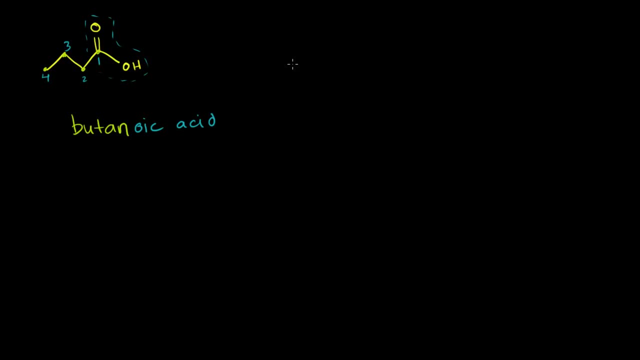 Let's do another one. Let's say we had something that looked like this. Let me put another one. Let's put another carbon on there, just like that, And let's say that there's a methyl group right over there. Now, clearly a carboxylic acid, but to name it systematically, 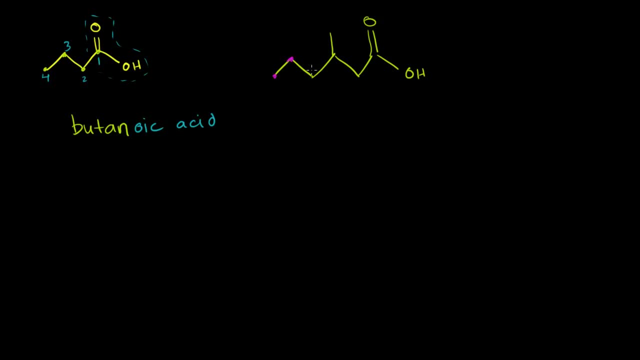 we just want to find the longest carbon chain. So we have one, two, three, four, five, six carbons. So our prefix will be hex. So it's hexan, It is hexan, And it's clearly not just a hexane. 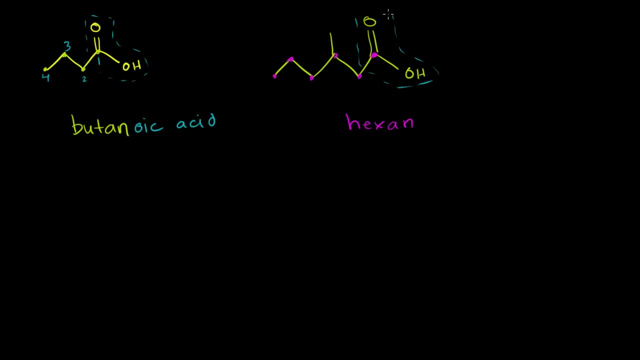 It's a hexanode. It's a hexanoic acid. It has this carboxyl group right here. This is hexanoic acid And we're not done because we still have this methyl carbon right over here And it is on the. we always want to start numbering. 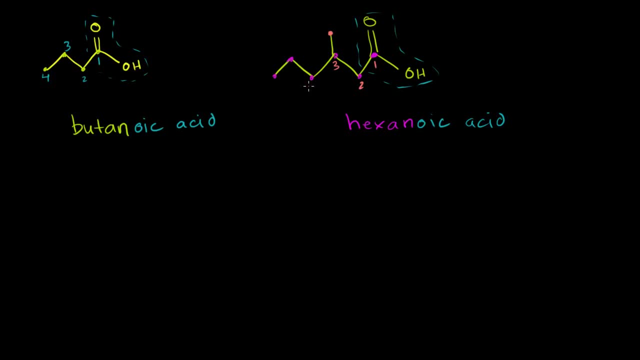 at this carbonyl carbon: one, two, three, four, five, six. It is at the number three, carbon. So this is three-methyl hexanoic acid. Let's do one more. Let's say we had a molecule that looked like this: 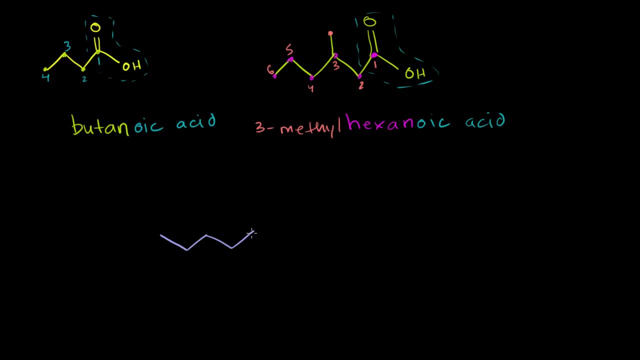 Let's see, That's one, two, three, four, five, six, seven carbons. And then we have our carboxyl group, just like that. And let's say that we had a double bond right over there. What would we call this? Well, once again, look for the longest carbon chain. We have one, two, three, four, five, six, Seven, Seven carbons, So the prefix is hept. Prefix is hept, So it's heptan. 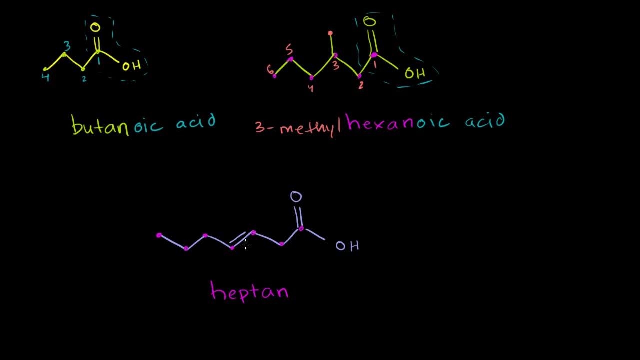 We won't just. and actually, let me be careful. This isn't an alkane. This has a double bond right here. This has a double bond right over here, So it's heptene. If this was just an alkane, we would just call it heptene. 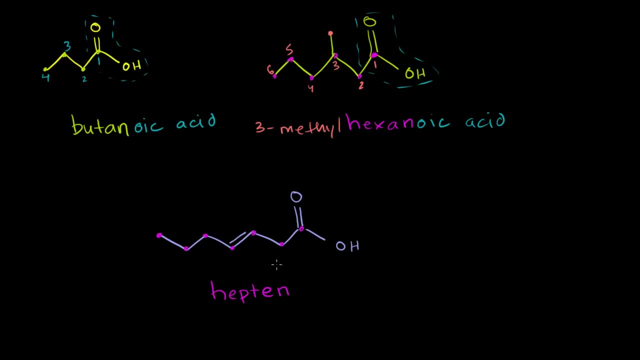 But we're not going to put this last e here, because this is a carboxylic acid. And to specify where that double bond is, we need to start numbering. And we start numbering at the carbonyl carbon one, two. 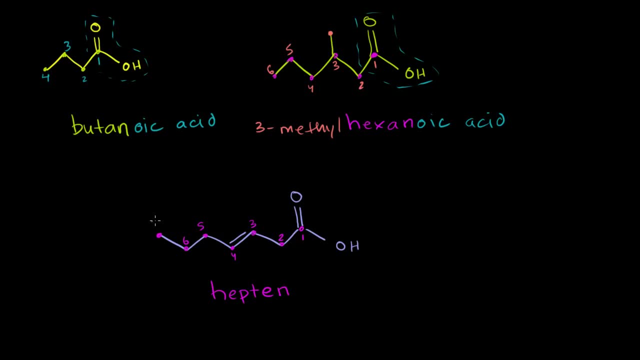 three, four, five, six, seven. So you could either name this 3-heptene- and I haven't finished it yet, I haven't put this final e over here- Or you could name it hept-3-ene, just like that.